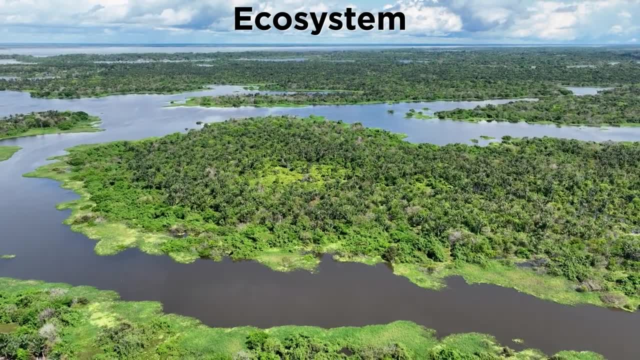 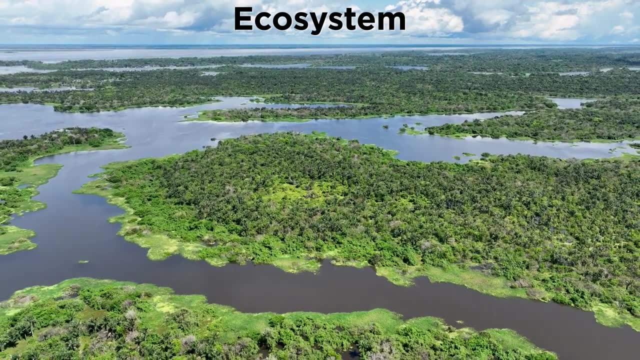 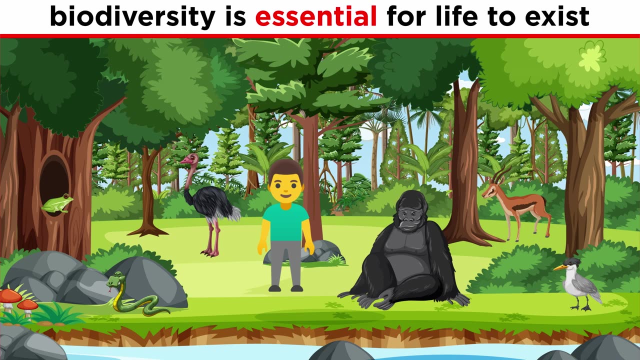 like bacteria. As we've been learning, each of these species and organisms work together in ecosystems, a complicated, intertwined web that somehow has to maintain balance and support life. Biodiversity is essential for the processes that support life, even human life, though sometimes we like to think of ourselves as separate from the natural world. 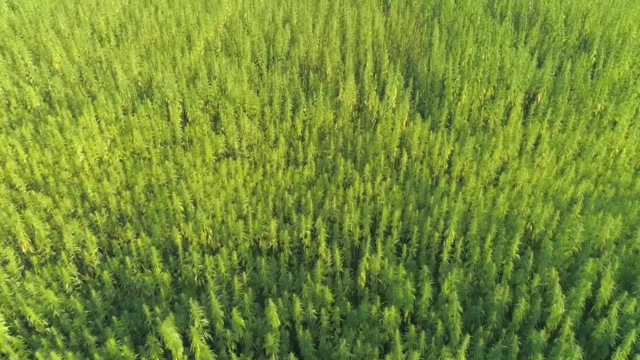 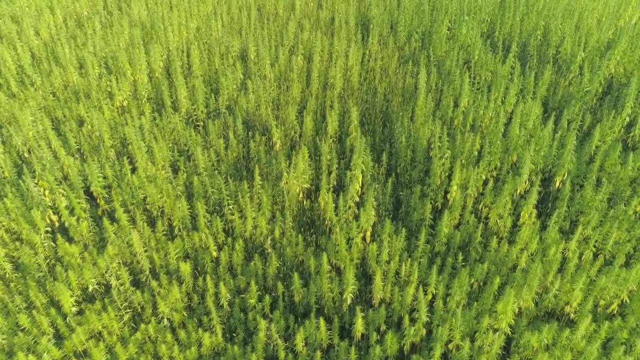 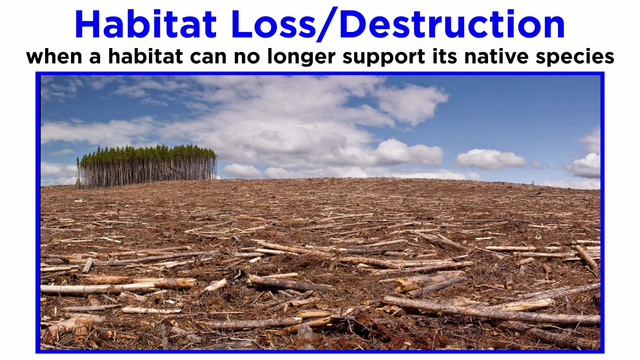 Without all the animals, plants and bacteria, we would not have the ecosystems that provide us with the air we breathe and the food we eat. So what are some of the most serious threats to biodiversity that we need to be aware of? Habitat loss or destruction is the process by which a natural habitat becomes incapable. 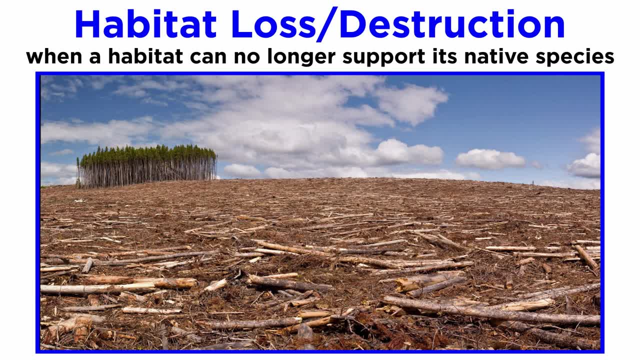 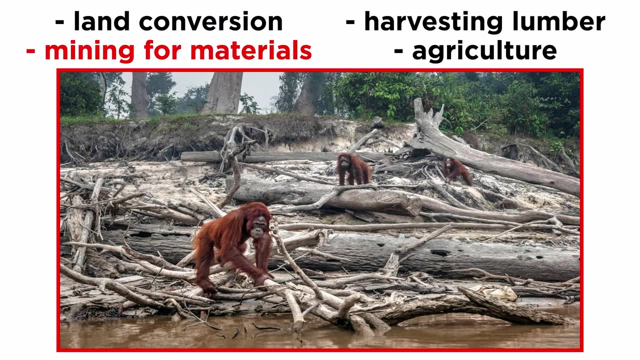 of supporting its native species. The organisms that previously inhabited the area are displaced or dead, leading to a reduction in biodiversity and species abundance. While there are many causes of habitat loss, land conversion for development due to growing populations, along with mining for materials, harvesting lumber and agriculture are at the top of the list. 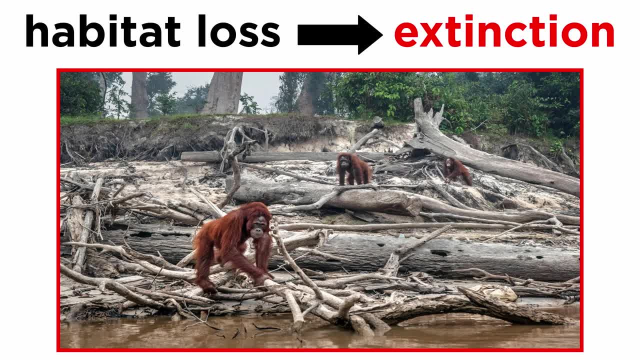 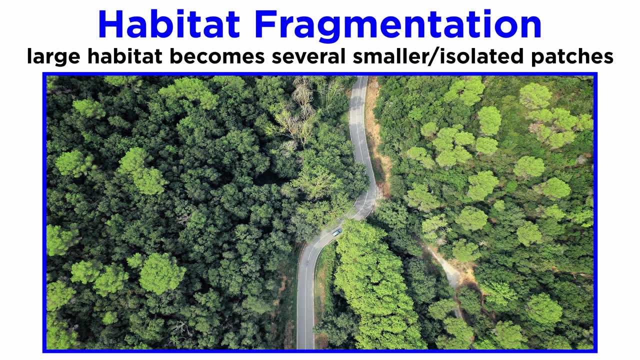 Loss of habitat can lead to the extinction of plants and animals. Habitat fragmentation is defined as the process by which a large expanse of habitat is transformed into a number of smaller patches of lesser total area, isolated from each other by a matrix of habitats. unlike 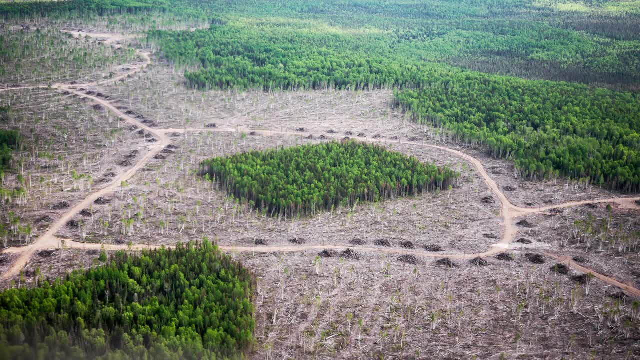 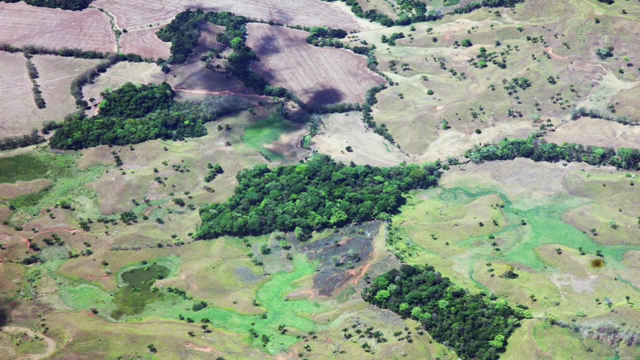 the original. In other words, habitats that were once continuous are now divided into separate fragments. This can happen when humans clear regions to build pasture or crop fields, and even the creation of hydrology Fragmentation can undermine the integrity of whole ecosystems by breaking up natural 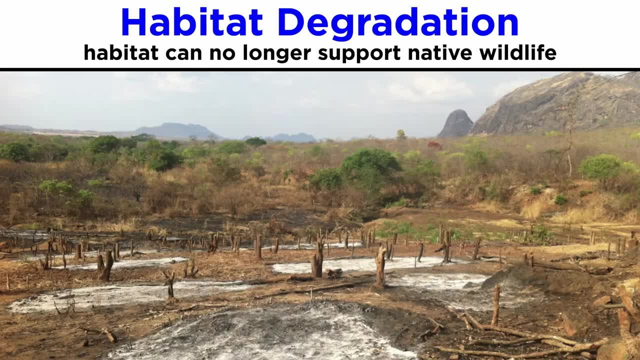 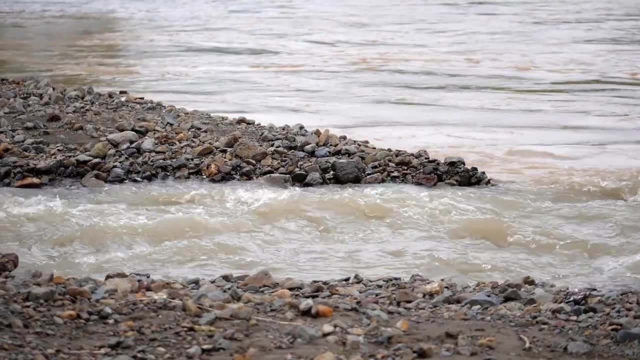 areas. Then there is habitat degradation. Pollution, invasive species and disruption of ecosystem processes, such as the changing intensity of fires, are some of the ways that habitats can become degraded, no longer supporting native wildlife. Another example of this is streams being degraded by runoff of sediments and chemicals from adjacent crop lands In 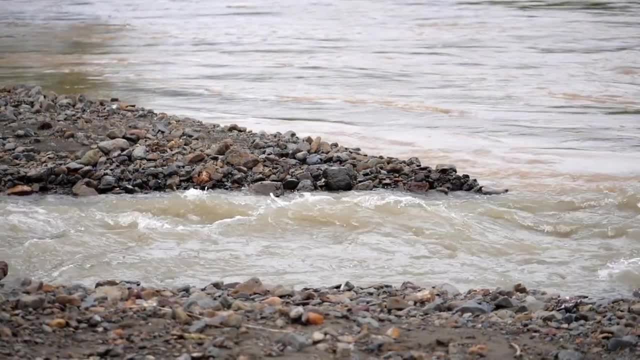 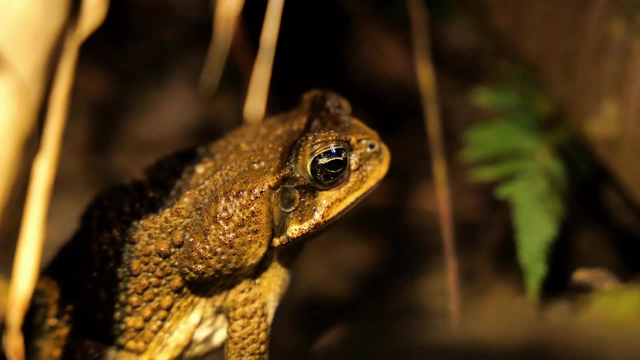 particular, there are many species that have been degraded by land or factories, leading to changes in the aquatic ecosystem. An invasive species is an organism that is not indigenous or native to a particular area. While not all non-native species are invasive, the ones 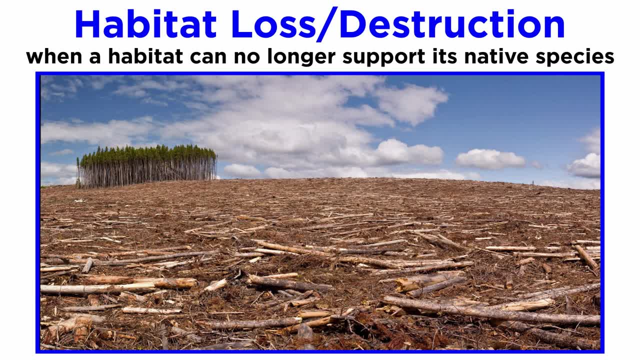 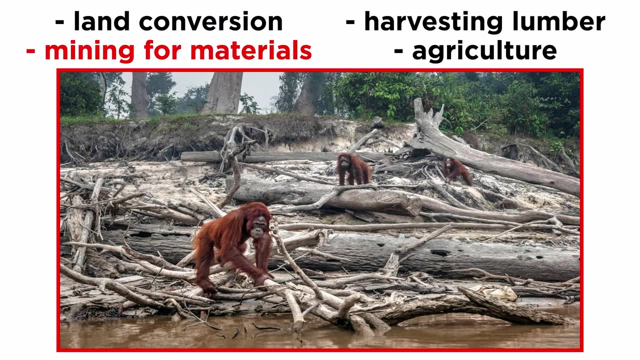 of supporting its native species. The organisms that previously inhabited the area are displaced or dead, leading to a reduction in biodiversity and species abundance. While there are many causes of habitat loss, land conversion for development due to growing populations, along with mining for materials, harvesting lumber and agriculture are at the top of the list. 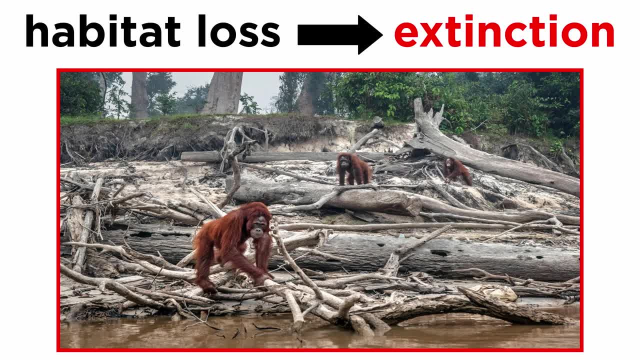 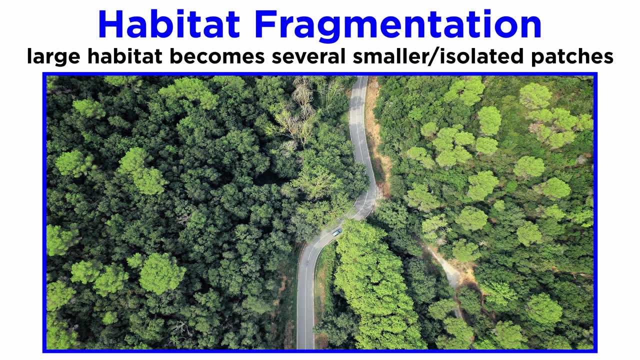 Loss of habitat can lead to the extinction of plants and animals. Habitat fragmentation is defined as the process by which a large expanse of habitat is transformed into a number of smaller patches of lesser total area, isolated from each other by a matrix of habitats. unlike 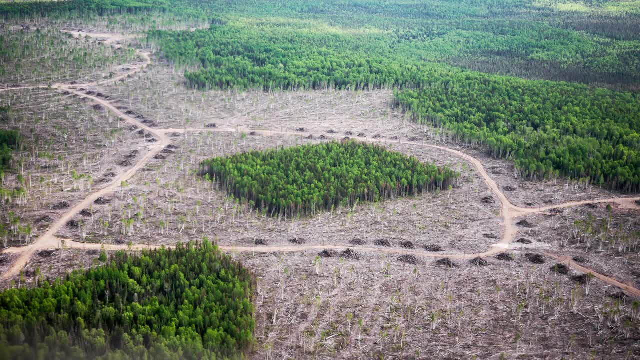 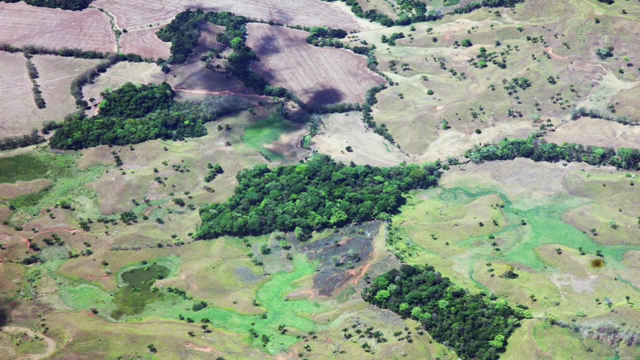 the original. In other words, habitats that were once continuous are now divided into separate fragments. This can happen when humans clear regions to build pasture or crop fields, and even the creation of hydrology Fragmentation can undermine the integrity of whole ecosystems by breaking up natural 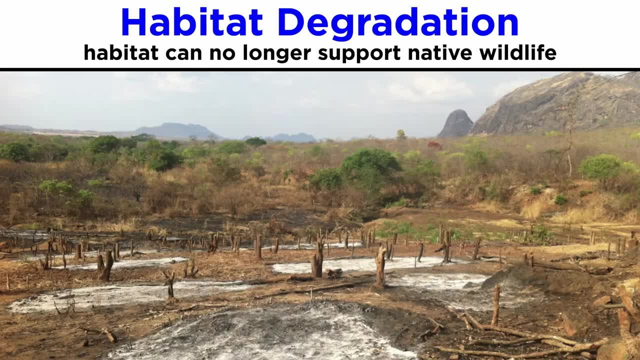 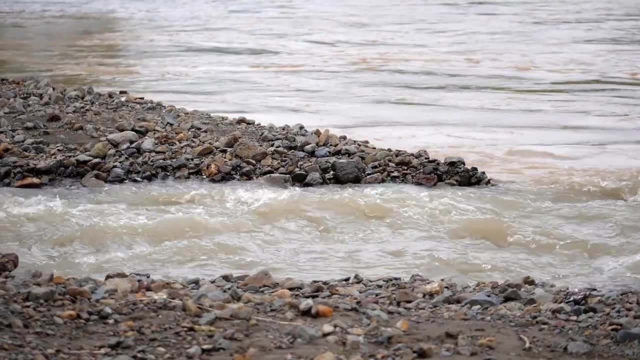 areas. Then there is habitat degradation. Pollution, invasive species and disruption of ecosystem processes, such as the changing intensity of fires, are some of the ways that habitats can become degraded, no longer supporting native wildlife. Another example of this is streams being degraded by runoff of sediments and chemicals from adjacent crop lands In 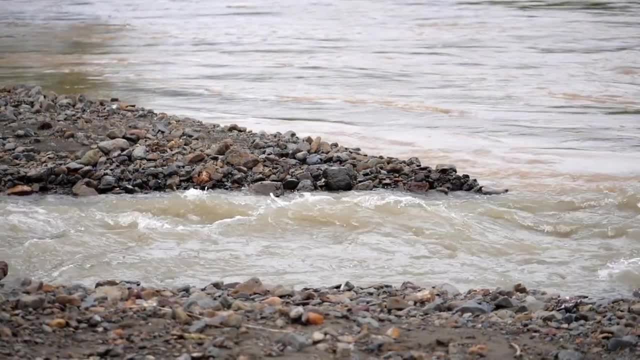 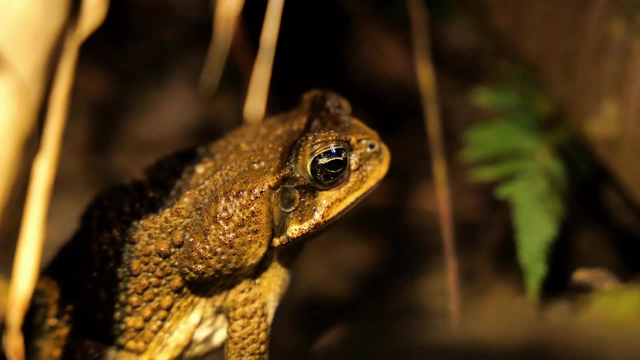 particular, there are many species that have been degraded by land or factories, leading to changes in the aquatic ecosystem. An invasive species is an organism that is not indigenous or native to a particular area. While not all non-native species are invasive, the ones 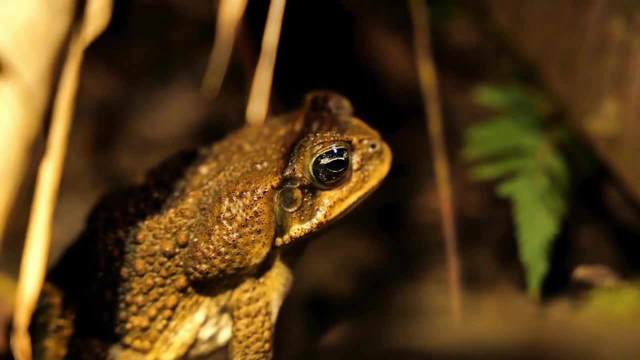 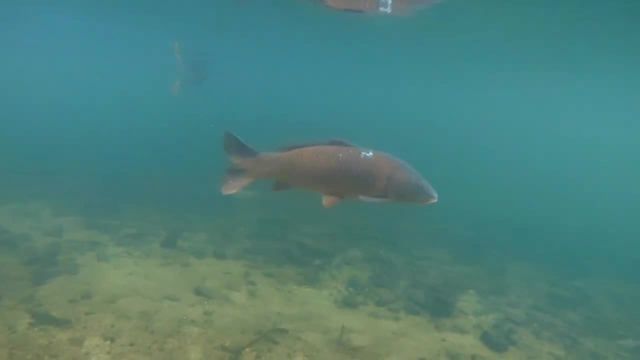 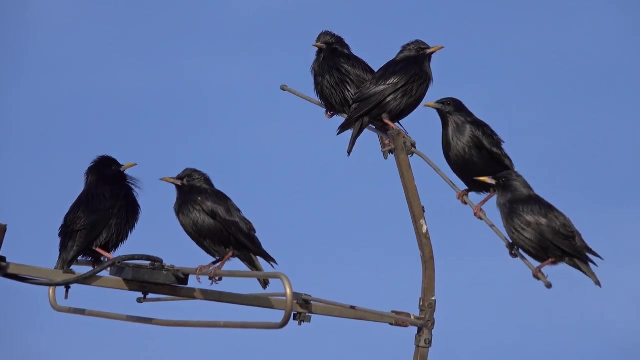 that are classified as such can cause great economic and environmental harm to an area. Some species may arrive in new areas through natural migration, perhaps prompted by changing temperature and precipitation conditions, but often they are introduced by the activities of other species. Why is this a problem? Invasive species are capable of causing extinctions in native plants. 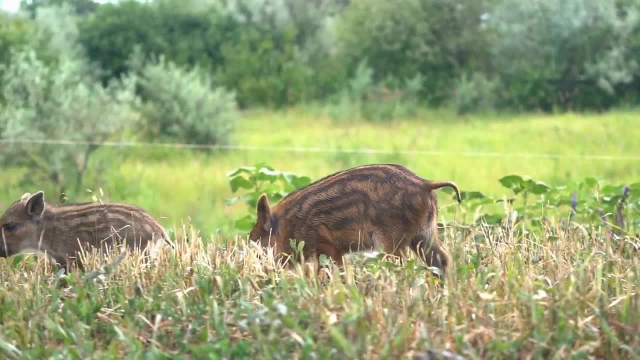 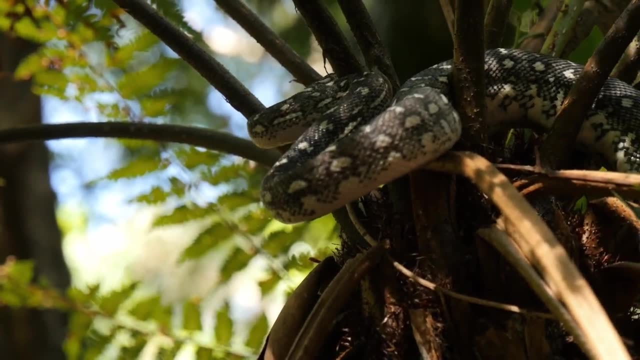 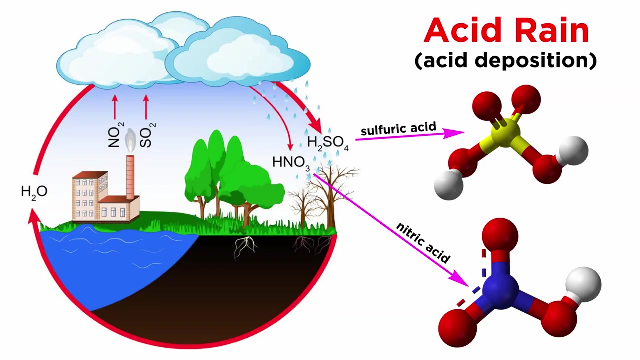 and animals by out-competing them for resources or preying on them incessantly. Their loss from the environment reduces biodiversity and may even alter the habitat, making it physically unsustainable for other species. Invasive species are among the leading threats to native wildlife. 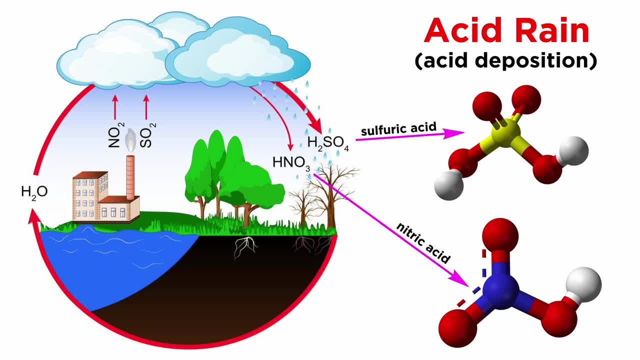 Another degradative phenomenon is acid rain or acid deposition, which is any form of precipitation with acidic components. Invasive species are among the leading threats to native wildlife. Another degradative phenomenon is acid rain or acid deposition, which is any form of precipitation with acidic components. 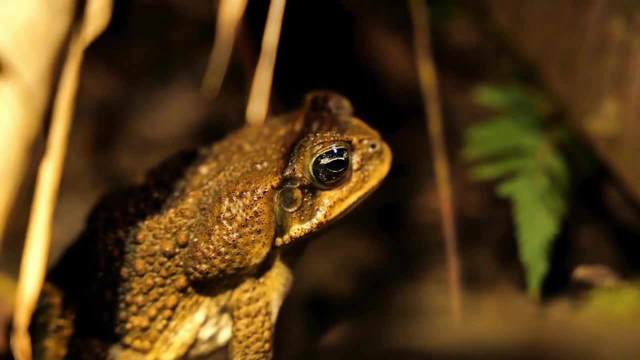 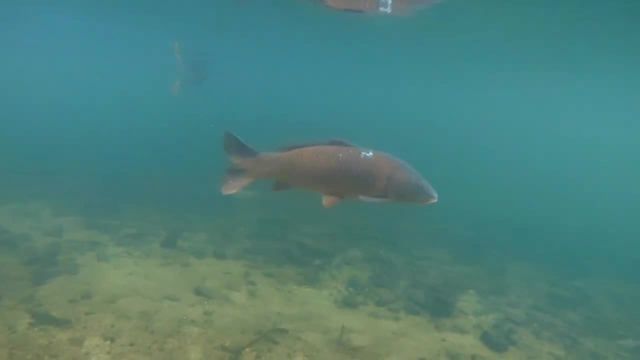 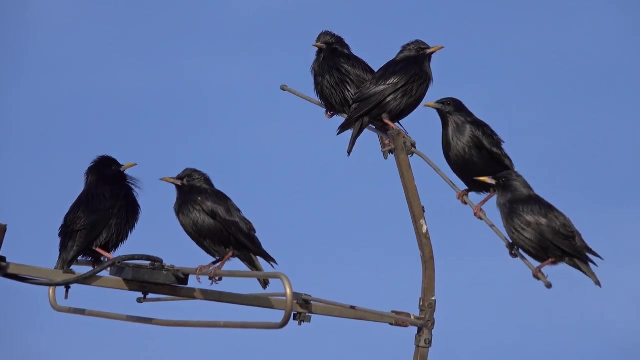 that are classified as such can cause great economic and environmental harm to an area. Some species may arrive in new areas through natural migration, perhaps prompted by changing temperature and precipitation conditions, but often they are introduced by the activities of other species. Why is this a problem? Invasive species are capable of causing extinctions in native plants. 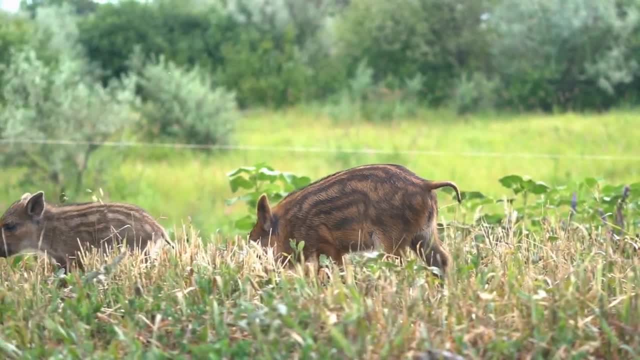 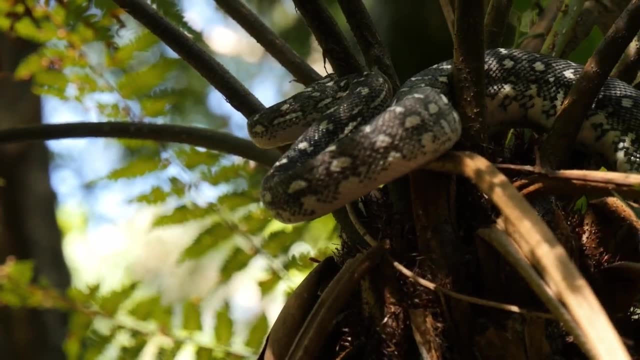 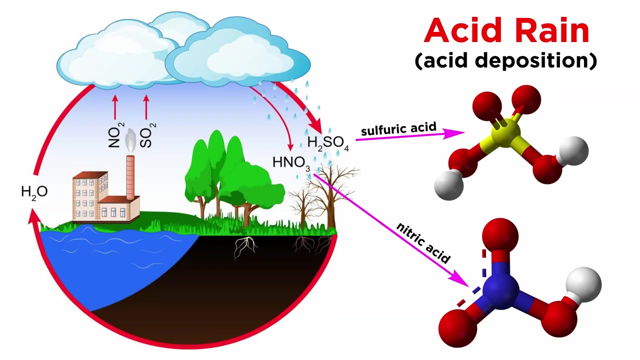 and animals by out-competing them for resources or preying on them incessantly. Their loss from the environment reduces biodiversity and may even alter the habitat, making it physically unsustainable for other species. Invasive species are among the leading threats to native wildlife. Another degradative phenomenon is acid rain or acid deposition, which is 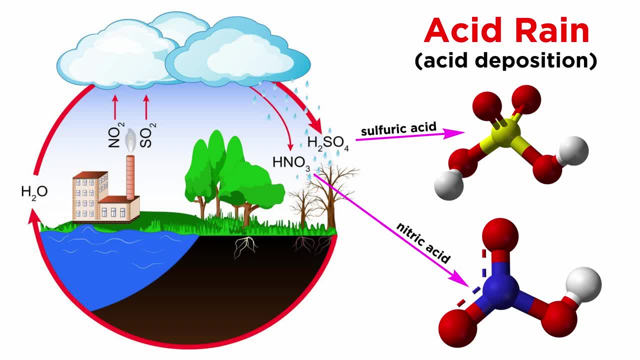 any form of precipitation with acidic components. Invasive species are among the leading threats to native wildlife. Another degradative phenomenon is acid rain or acid deposition, which is any form of precipitation with acidic components, like sulfuric or nitric acid, that falls to the ground. It can include rain, snow, fog. 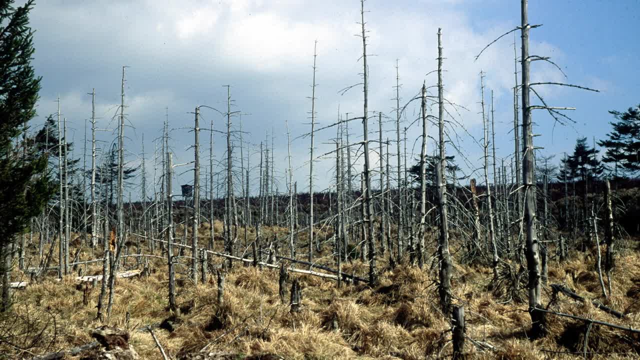 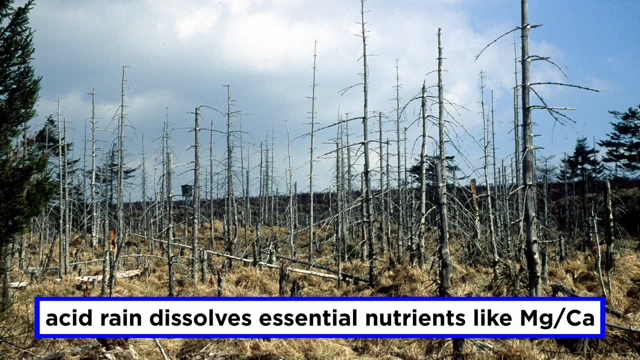 hail or even dust. Acid rain can be extremely harmful to forests. The rain seeps into the ground, dissolving nutrients such as magnesium and calcium that the trees need to grow. Additionally, acid rain can cause aluminum to be released into the soil, making it difficult for trees 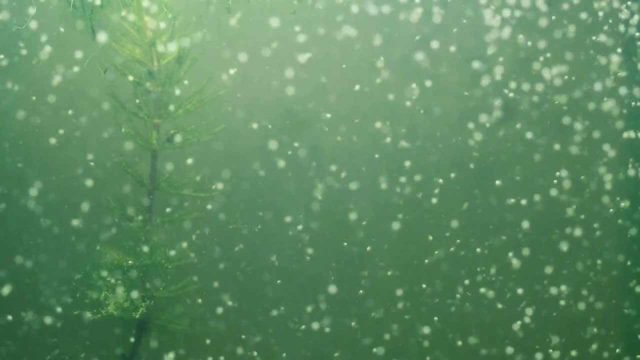 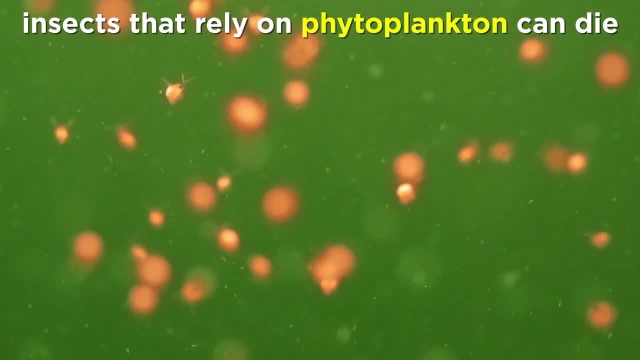 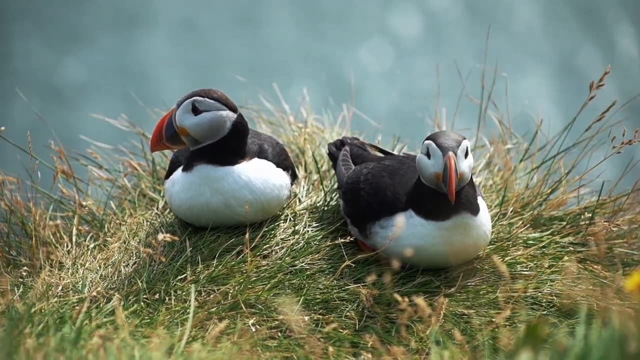 to die. Insects, which rely on the phytoplankton for food, now have less food, and they begin to die. Birds reliant on insects for food now also have less food, and so on, creating disturbances all the way up the food web. 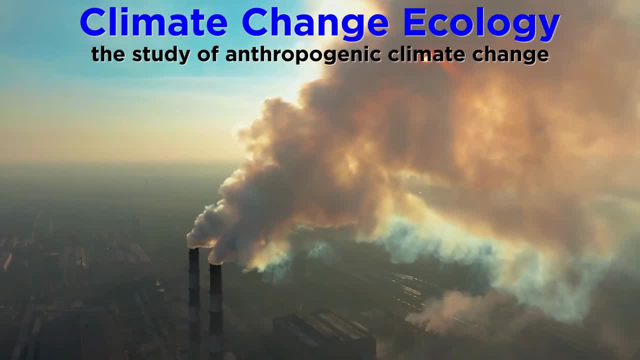 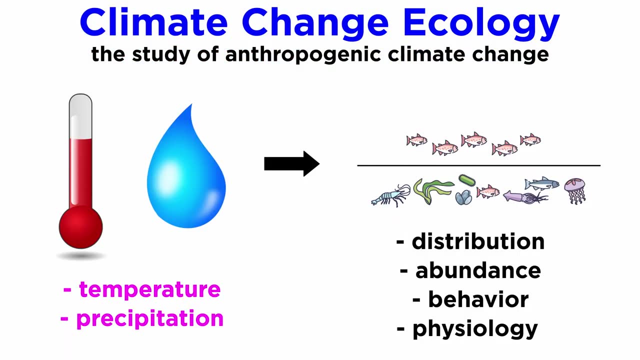 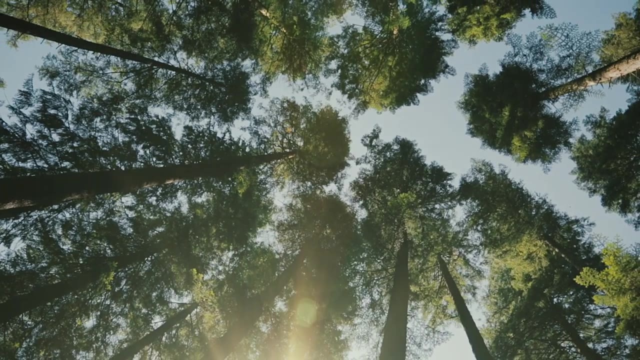 Next climate change ecology is the study of the effects of anthropogenic, human-caused climate change on any aspect of ecology. This includes the effects of altered temperature and precipitation on the distribution, abundance, behavior and physiology of populations and communities. In addition to altering plant communities, climate change likely will 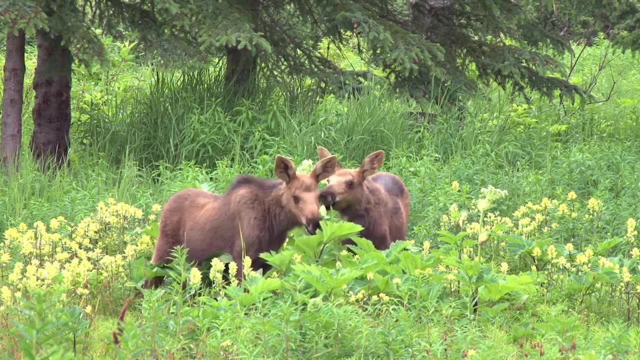 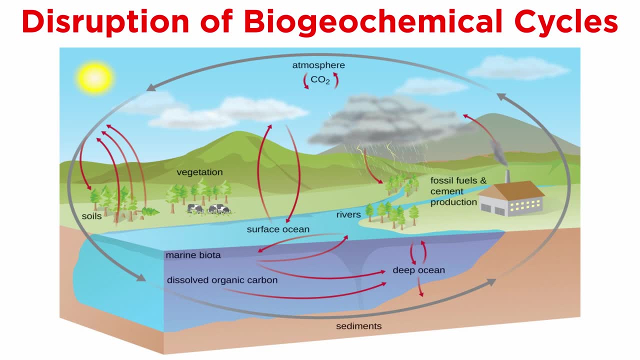 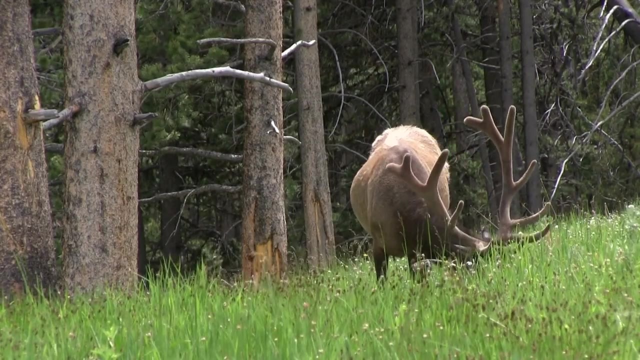 also disrupt the ecological balance between interdependent and often endangered plant and animal species. Biodiversity will be reduced and Earth's water, energy, carbon and other element cycles will be disrupted, leading to vast ecological stress. Climate change is one of the biggest threats that wildlife is facing. At what point is irreparable harm? 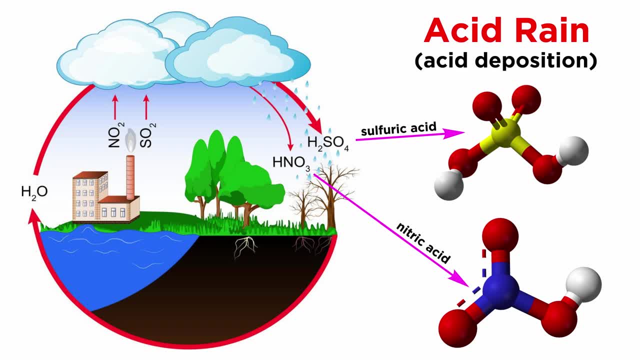 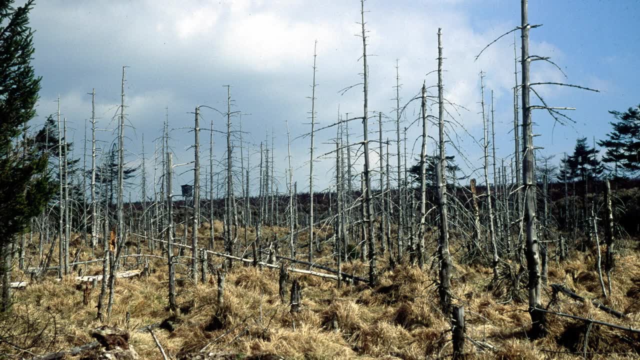 acid deposition, which is any form of precipitation with acidic components, like sulfuric or nitric acid, that falls to the ground. It can include rain, snow, fog, hail or even dust. Acid rain can be extremely harmful to forests. The rain seeps into the ground, dissolving nutrients. 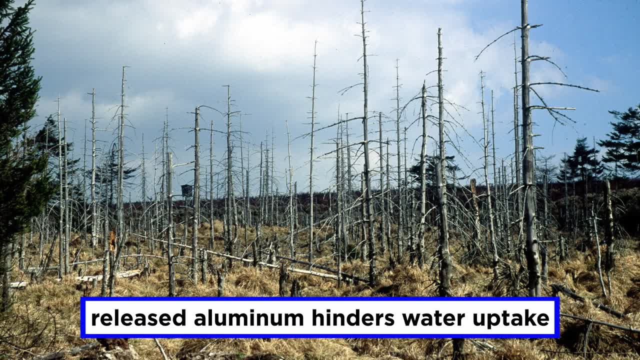 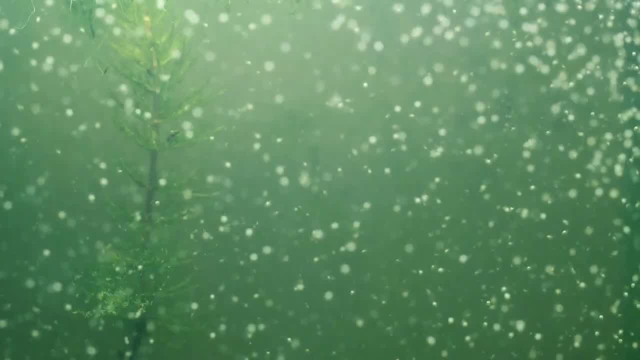 such as magnesium and calcium, that the trees need to grow. Additionally, acid rain can cause aluminum to be released into the soil, making it difficult for trees to take up water. In aquatic environments, acid rain can cause phytoplankton to die. Acid rain can cause. 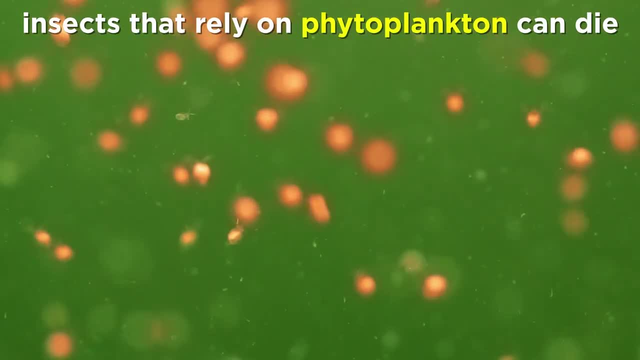 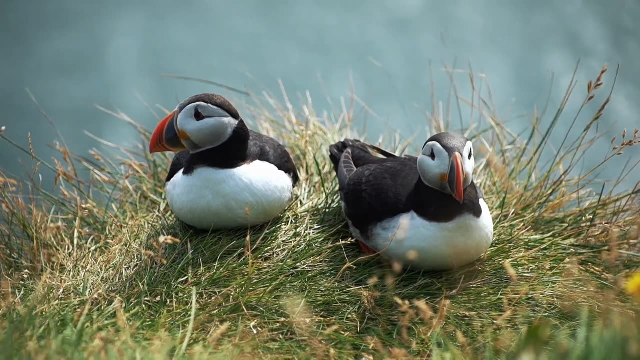 phytoplankton to die. Insects which rely on the phytoplankton for food now have less food, and they begin to die. Birds reliant on insects for food now also have less food, and so on, creating disturbances all the way up the food web. 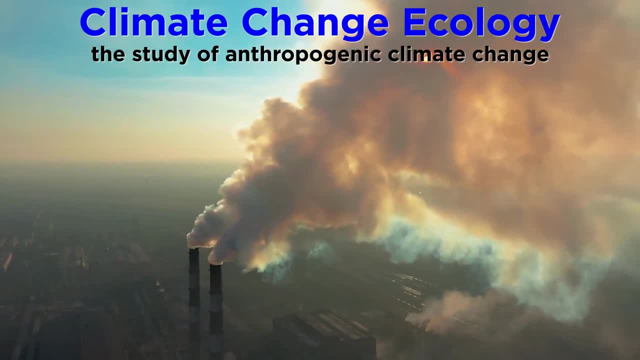 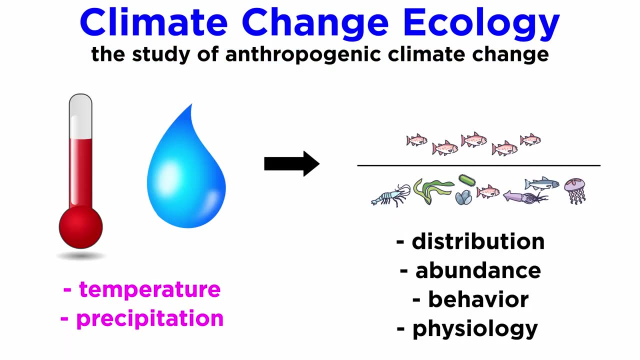 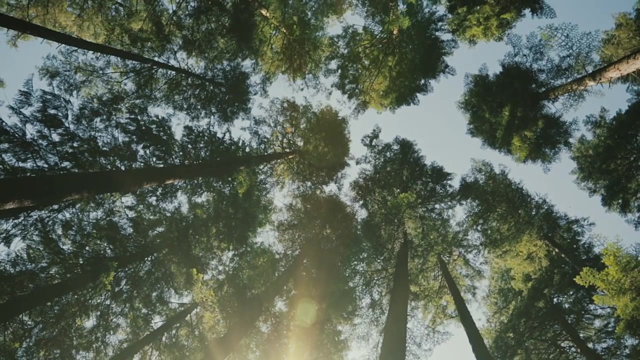 Next climate change ecology is the study of the effects of anthropogenic, human-caused climate change on any aspect of ecology. This includes the effects of altered temperature and precipitation on the distribution, abundance, behavior and physiology of populations and communities. In addition to altering plant communities, climate change likely will 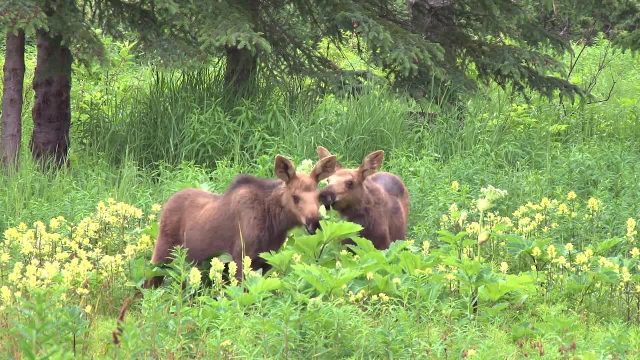 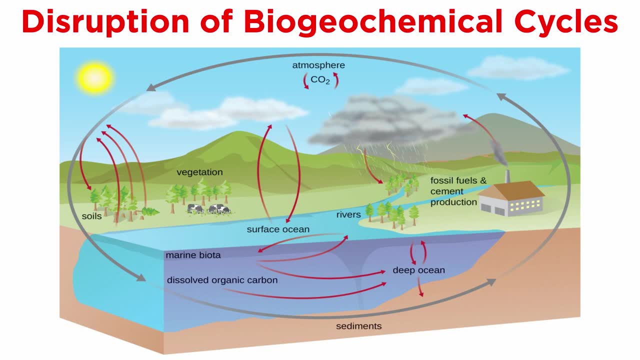 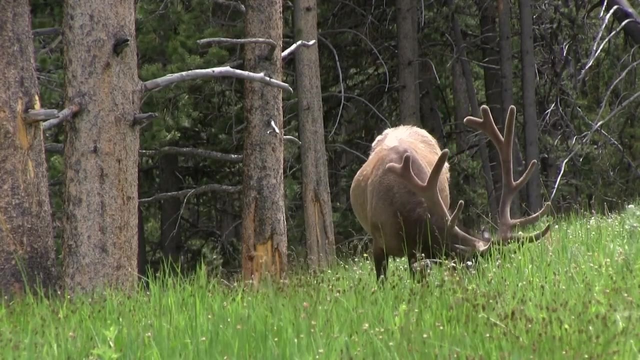 also disrupt the ecological balance between interdependent and often endangered plant and animal species. Biodiversity will be reduced and Earth's water, energy, carbon and other element cycles will be disrupted, leading to vast ecological stress. Climate change is one of the biggest threats that wildlife is facing. At what point is irreparable harm? 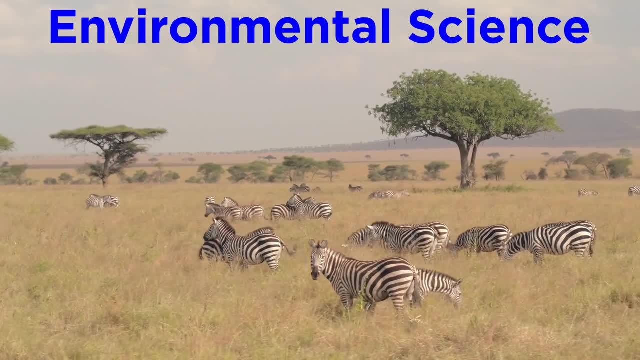 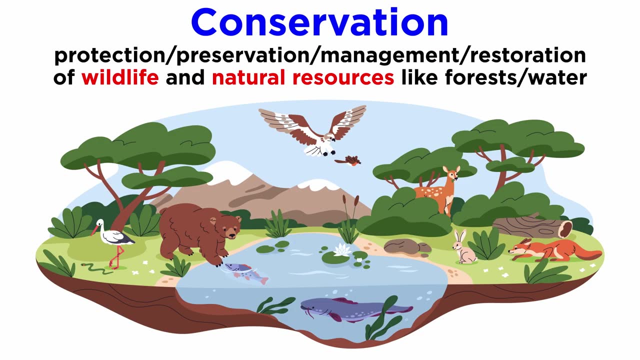 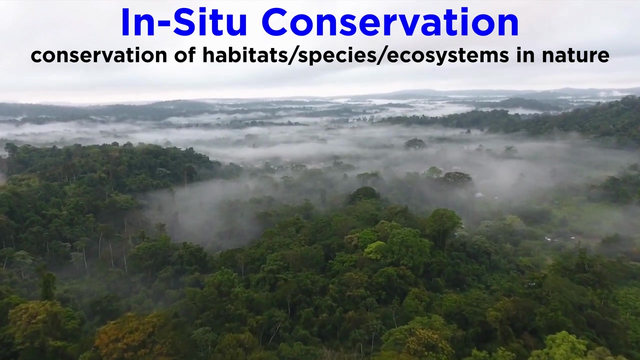 done. We will return to this very important question in detail and potential solutions in the upcoming series on environmental science. In the meantime, conservation is the protection, preservation, management or restoration of wildlife and natural resources such as forests and water. In situ, conservation includes the conservation of habitats, species and ecosystems, where 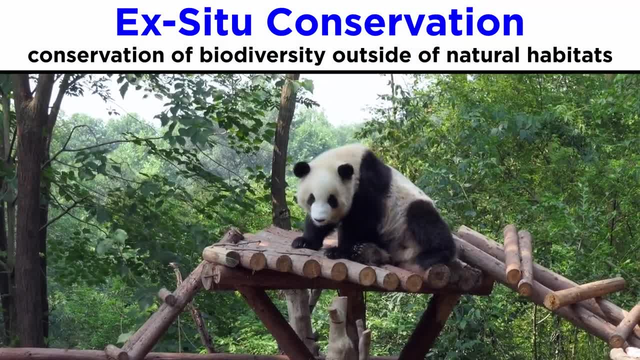 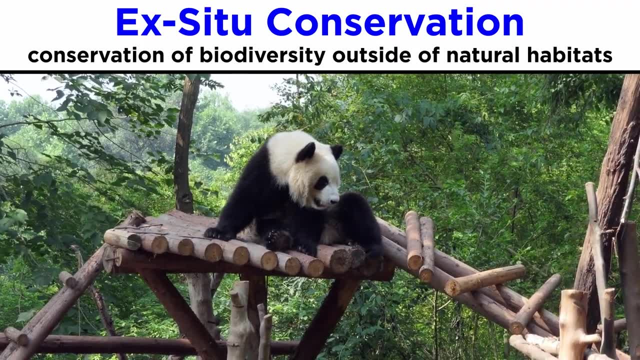 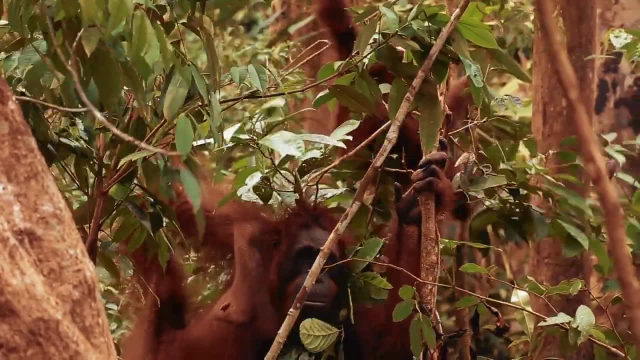 they naturally occur. Ex situ refers to the conservation of elements of biodiversity outside of the context of natural habitats. Examples of this include zoos and seed banks. Both of these types of conservation are important. Sometimes. in situ conservation is not always possible, as habitats are too degraded or there may be competition for land. meaning: 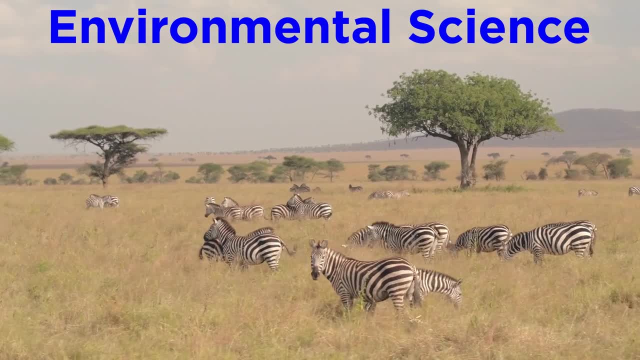 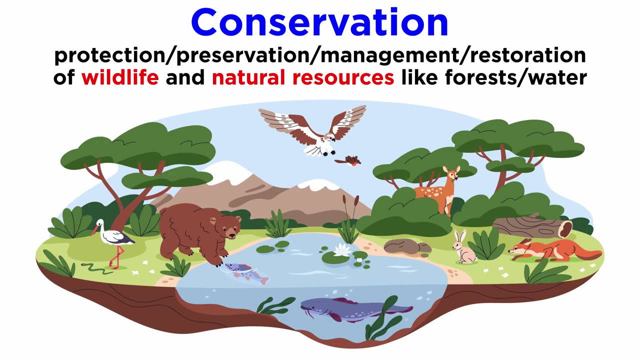 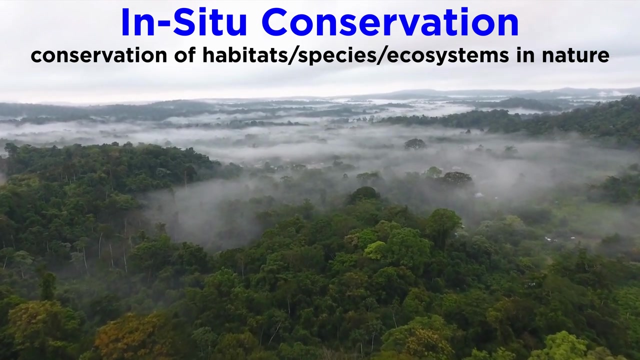 done. We will return to this very important question with more detail and potential solutions in the upcoming series on environmental science. In the meantime, conservation is the protection, preservation, management or restoration of wildlife and natural resources such as forests and water. In situ, conservation includes the conservation of habitats, species and ecosystems, where 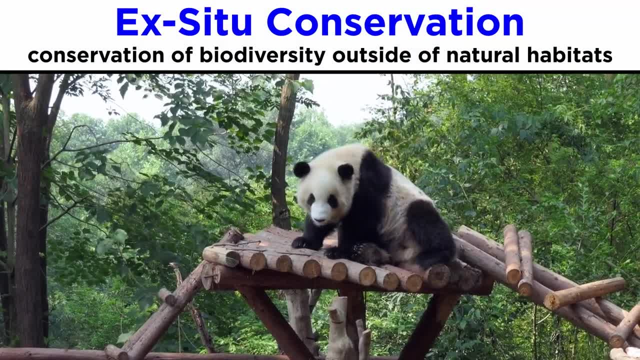 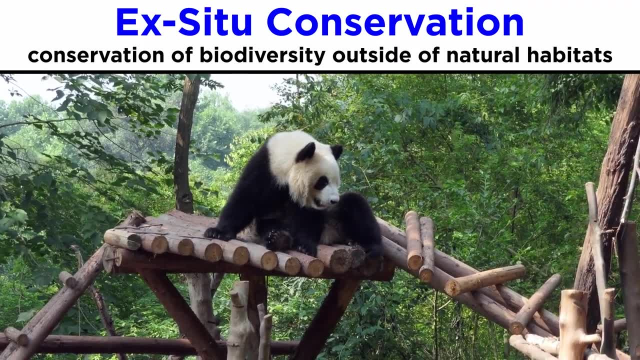 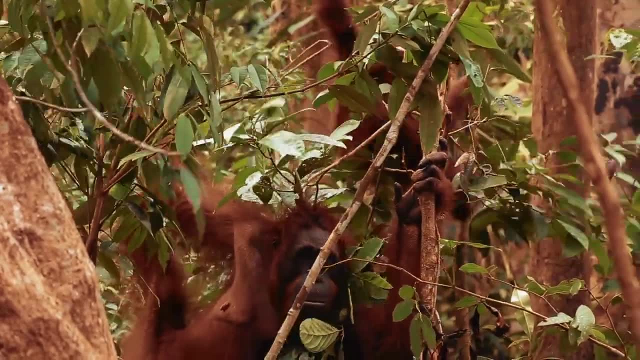 they naturally occur. Ex situ refers to the conservation of elements of biodiversity out of the context of natural habitats. Examples of this include zoos and seed banks. Both of these types of conservation are important. Sometimes in situ conservation is not always possible, as habitats are too degraded or there may be competition for land, meaning species. 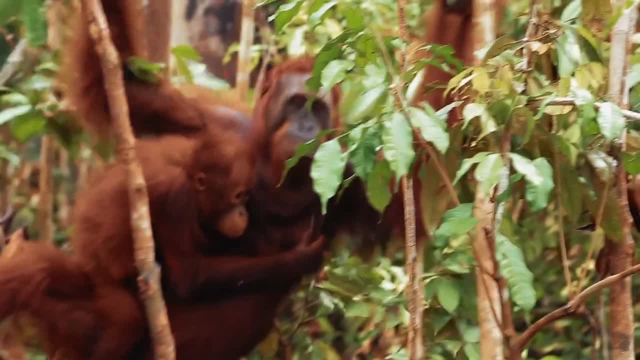 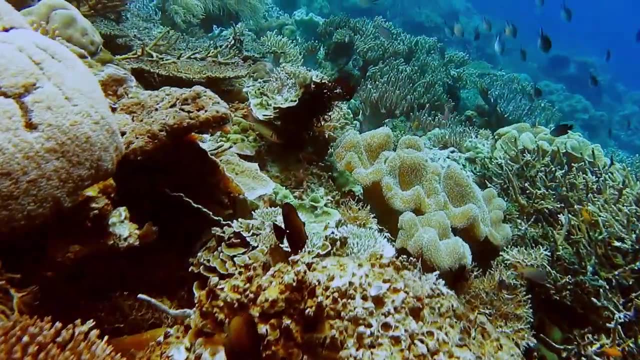 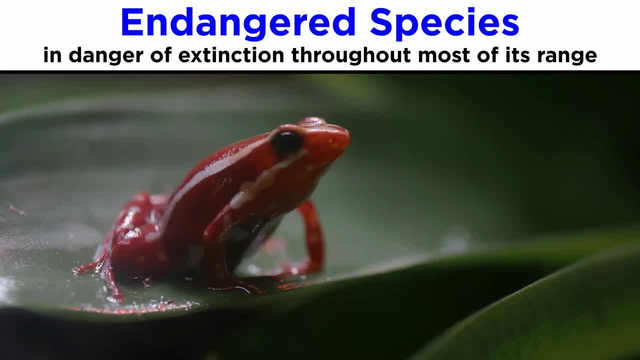 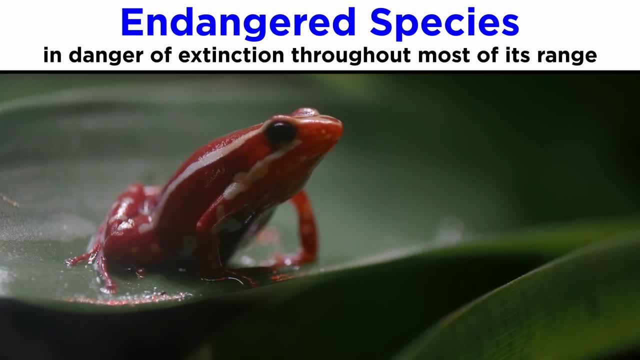 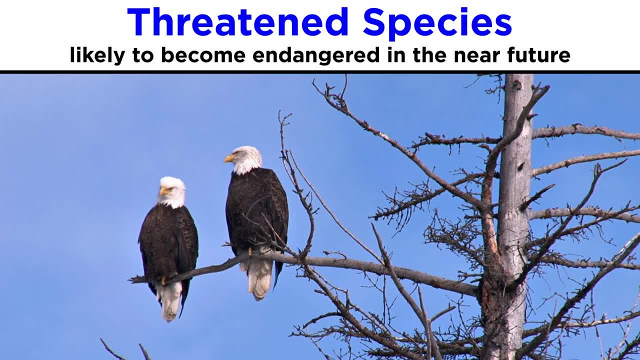 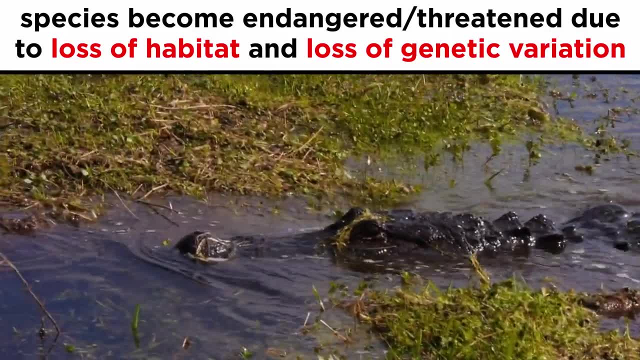 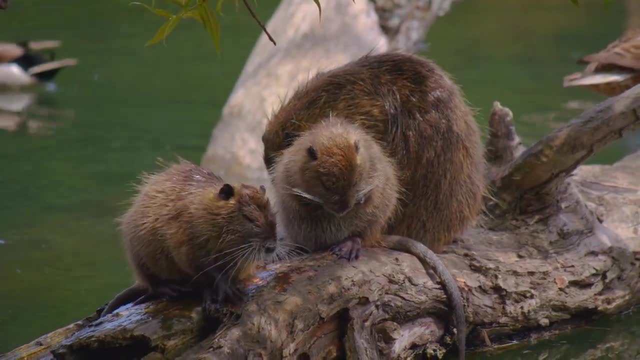 its geographical range Threatened means a species is likely to become endangered within the foreseeable future. Species become threatened or endangered for two main reasons: loss of habitat and the loss of genetic variation. Invasive species play a large role in threatening or endangering species as well, especially. 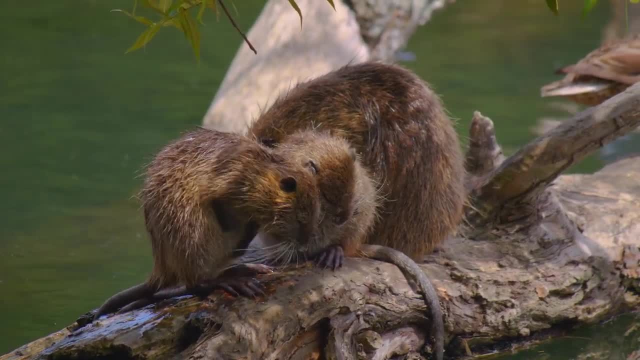 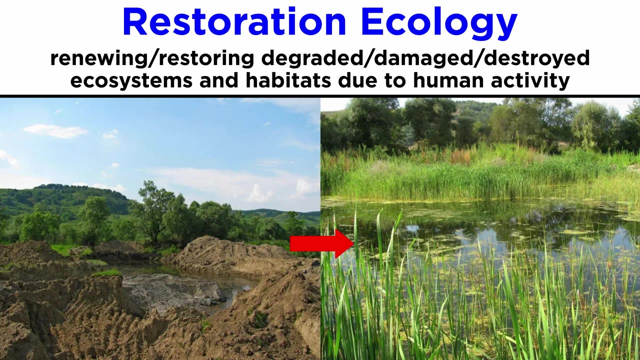 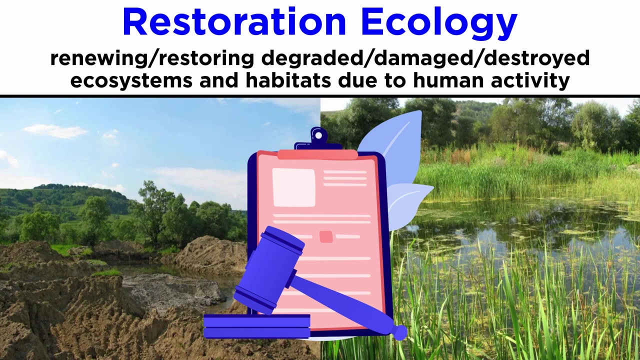 as native species may be much closer to adapting to new climatic conditions than the invasive species that replace them. Restoration ecology is the scientific study supporting the practice of renewing or restoring degraded, damaged or destroyed ecosystems and habitats due to human activity. It is often the case that effective restoration requires an explicit goal or policy. 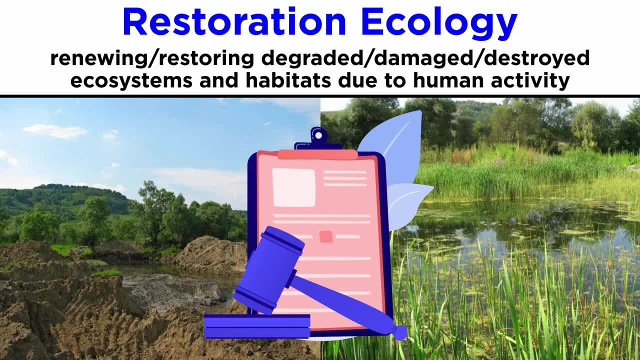 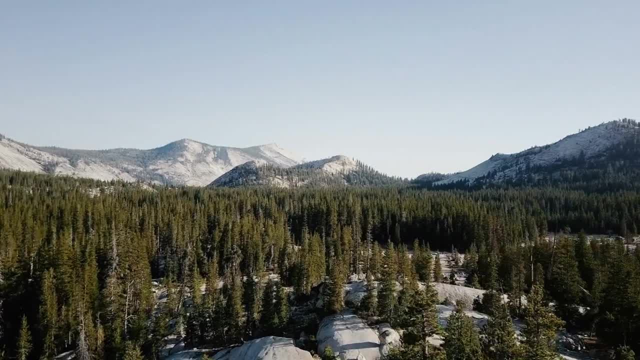 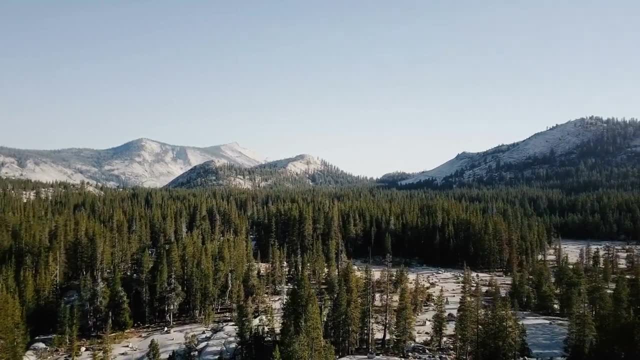 These goals reflect societal choices from competing policy priorities, and it can be challenging to instigate any kind of action. Nevertheless, it is in our best interest to continue trying, as ecosystems provide us with food, fuel and timber that we need to survive and thrive as a species. 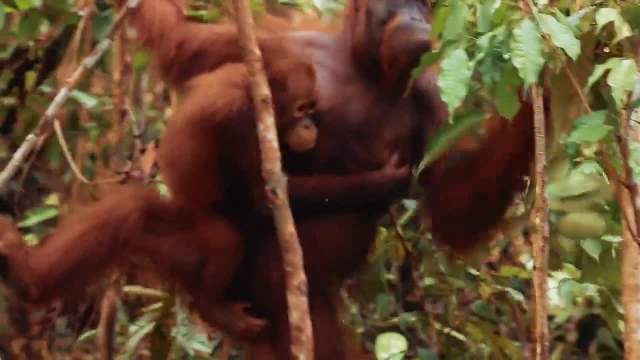 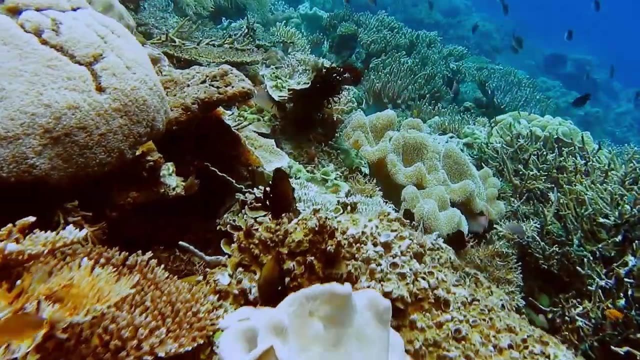 species need to be removed to save them. Orangutans in Indonesian rainforests are an example of this. Areas to conserve typically include hotspots of diversity and areas where there are threatened habitats or habitats that are not protected by the environment In situ. 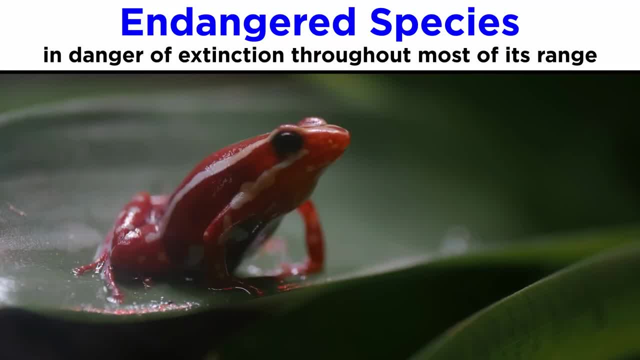 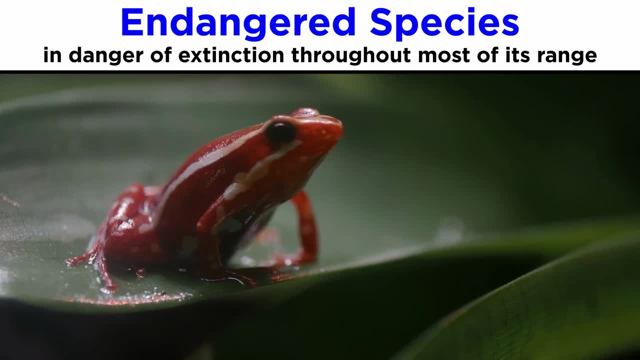 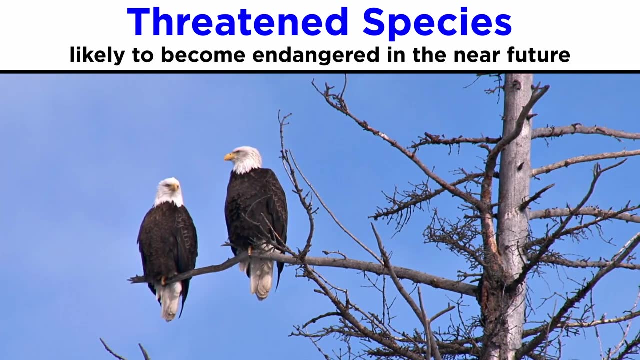 conservation includes the conservation of habitats or species which require restoration. Plants and animal species may be listed as endangered when in danger of extinction throughout all or a significant portion of its geographical range, Threatened means: a species is likely to become endangered within the foreseeable future. Species become threatened or endangered. 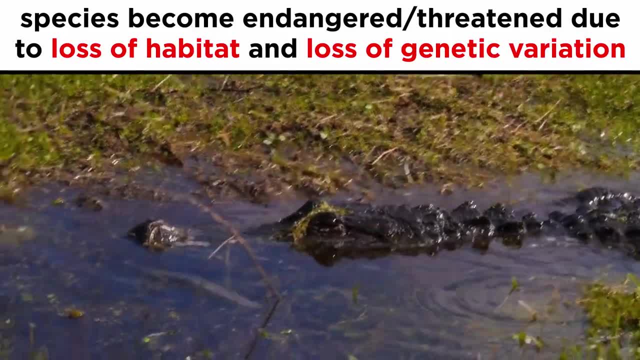 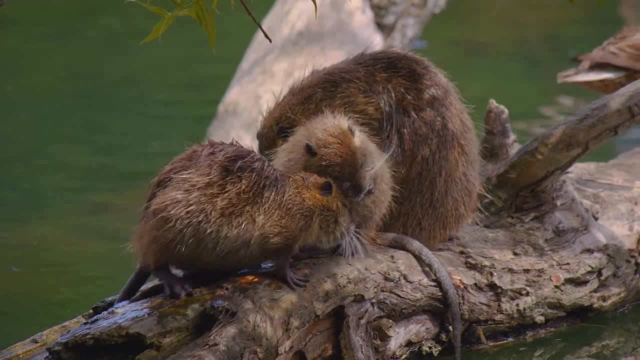 for two main reasons: loss of habitat and the loss of genetic variation. Invasive species play a large role in threatening or endangering species as well, especially when they are not protected by the environment. These species may be much closer to adapting to new climatic. 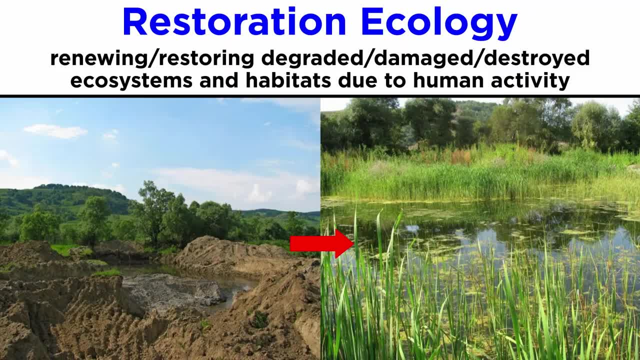 conditions than the invasive species that replace them. Restoration ecology is the scientific study supporting the practice of renewing or restoring degraded, damaged or destroyed ecosystems and habitats due to human activity. It is often the case that effective restoration requires an explicit goal or policy. These 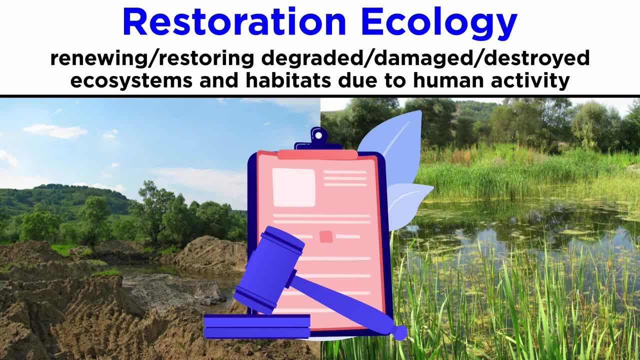 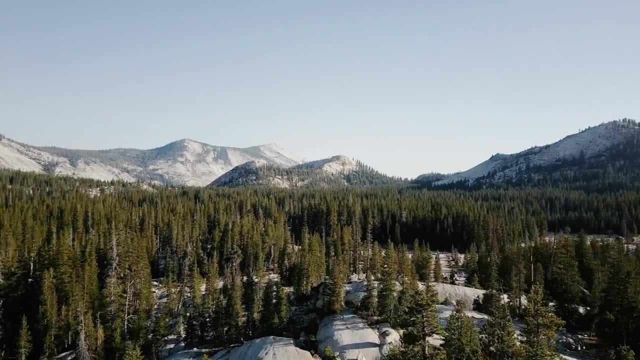 goals reflect societal choices from competing policy priorities, and it can be challenging to instigate any kind of action. Nevertheless, it is in our best interest to continue trying, as ecosystems provide us with food, fuel and timber that we need to survive and thrive. 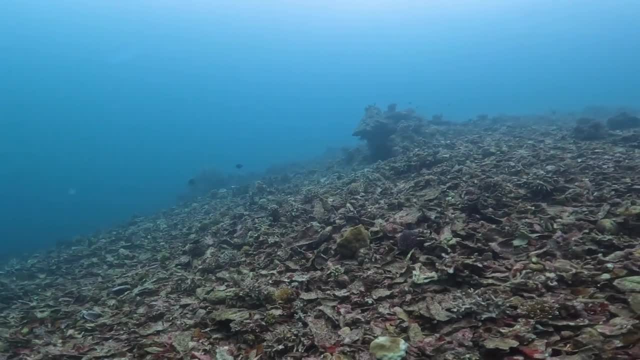 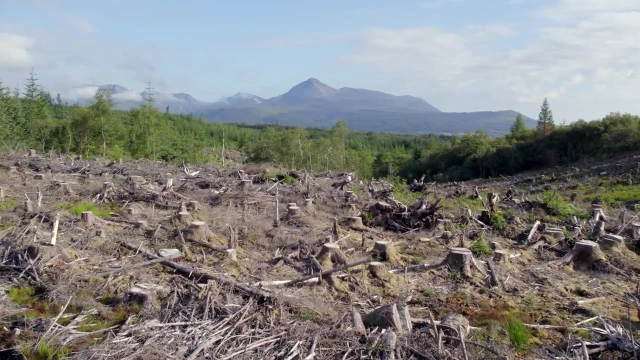 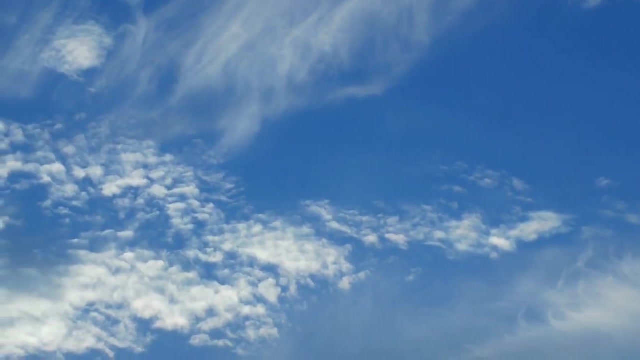 as a species. If we destroy it all, we destroy the ability to live in harmony with nature and to support our own human communities. Habitat losses and extinctions affect the entire planet, including us. Ecological restoration has many positives: the potential to improve. 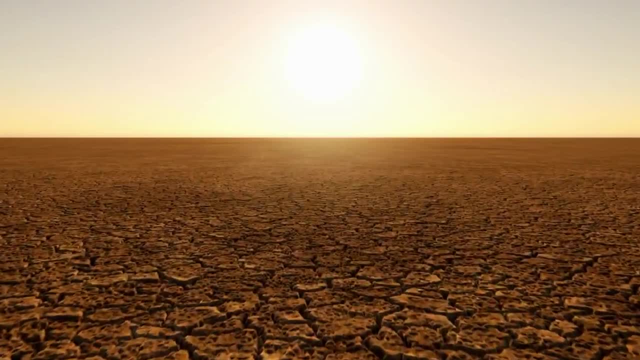 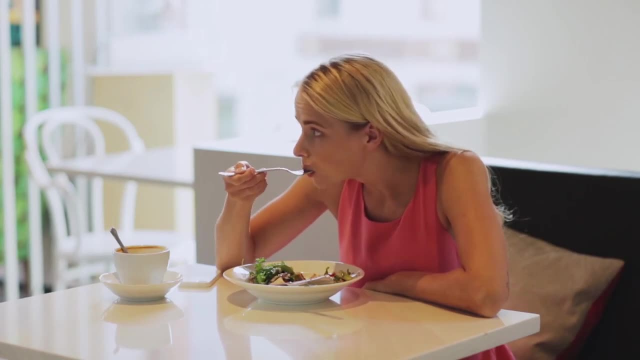 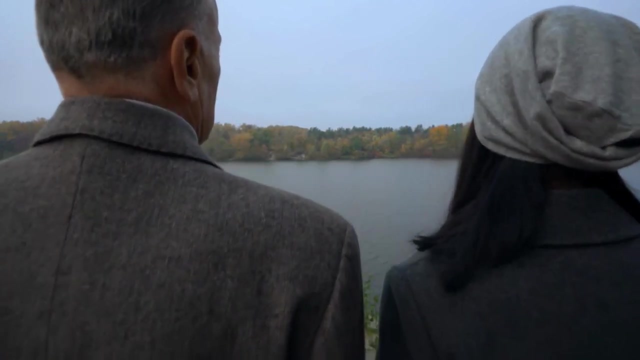 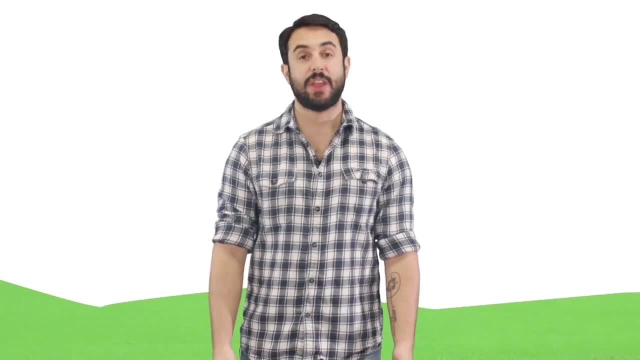 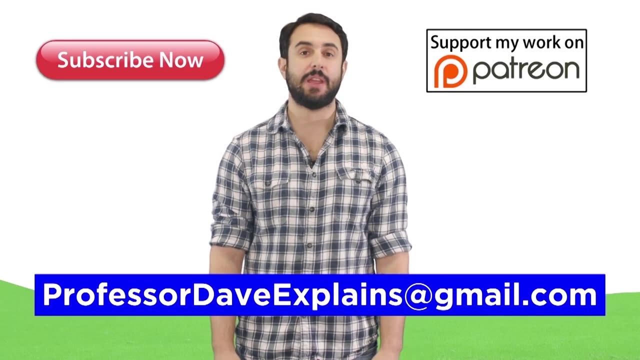 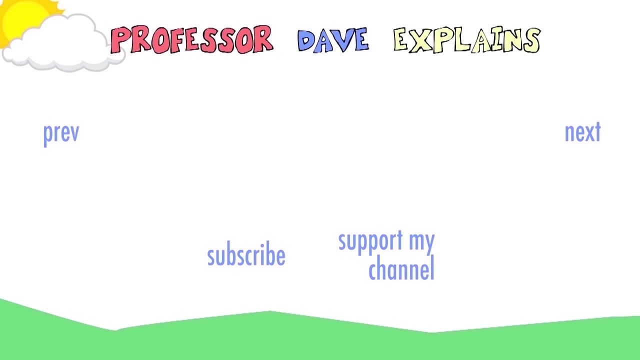 species and ourselves. Thank you for listening to this episode of Habitat for Humanity and I hope you enjoyed it. If you have any questions or comments, please feel free to ask them in the comments below.